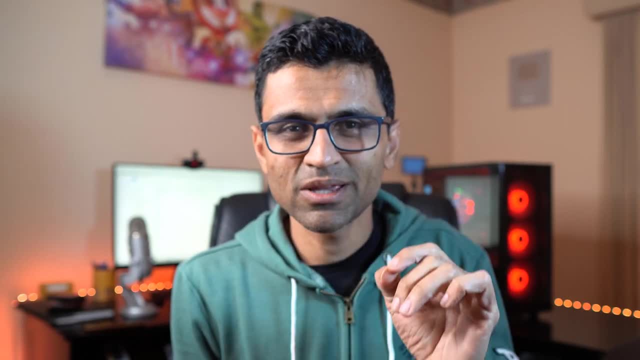 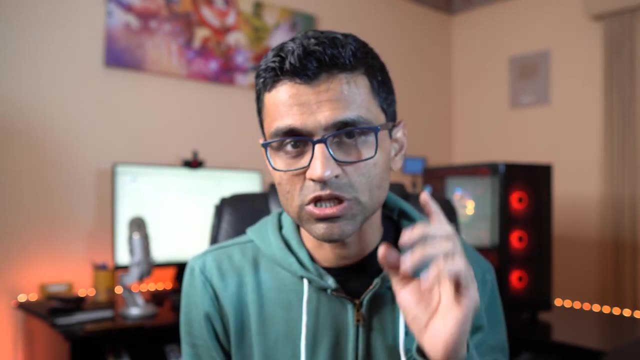 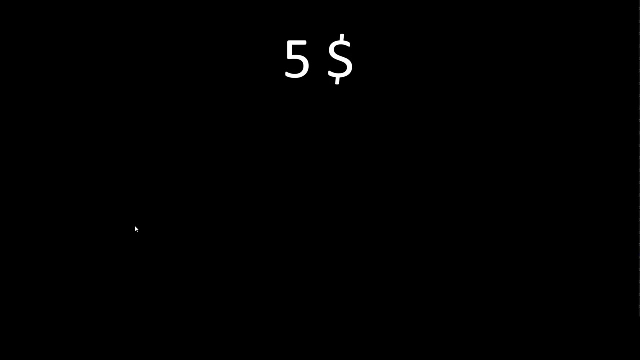 In a very simple language I will explain you what is log or logarithmic function and what is the significance of it in data science and machine learning. We'll also look at some Python code. Let's get started. Let's say I have $5 and I am putting that in a bank which gives me 5x return. 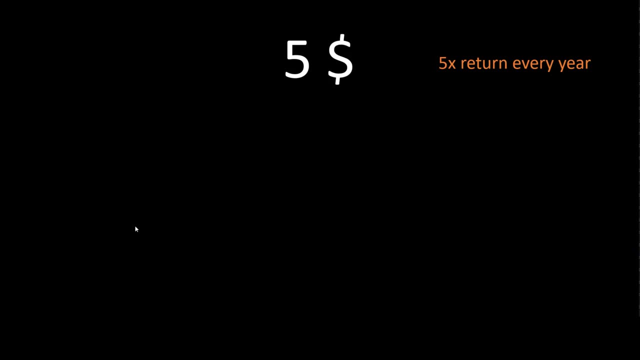 So if I put 5, it will give me 5x. If I put $7, it will give me 7x return. It's a magic bank, you know. very customer-friendly bank. After one year I will have $25.. After two years. 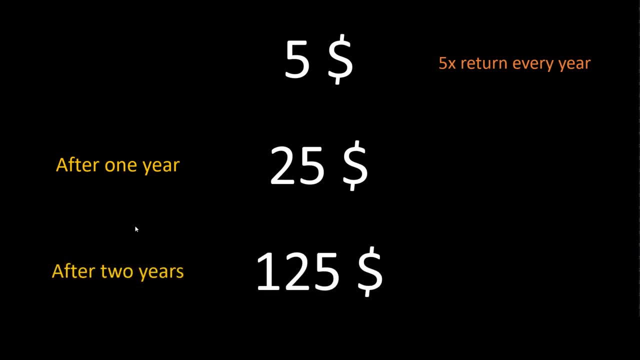 I will have $125 because every year it is being multiplied by 5x. To represent this concept, in mathematics you use something called exponent. So exponent meaning, 5 raised to 2 is 25, 5 raised to 3 is 125.. Now let me ask a different question, or rather a reverse question, where I have $125. 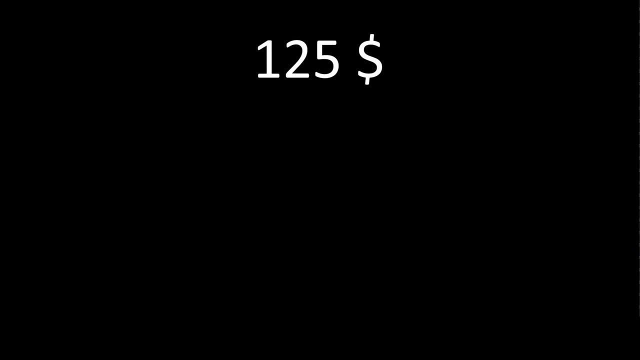 and I have $125.. So I have $125 and I have $125.. So I have $125 and I have $125.. So I have $125 today in my bank. I know that at some point I started with $5 base investment, but I don't know. 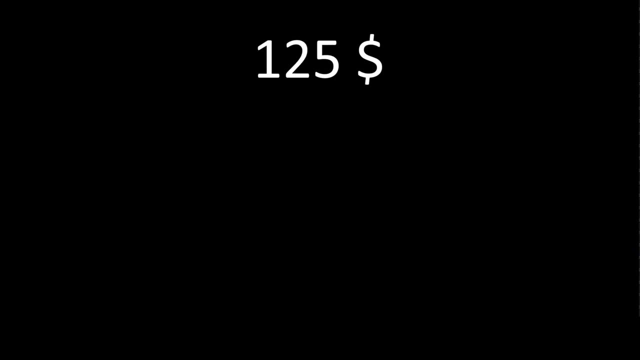 how many years it took to get to $125.. So how do you find that? So the question is again simple. I started with base investment of $5.. I know that bank is giving me 5x return, but I don't know how many years will it take to make that money $125. 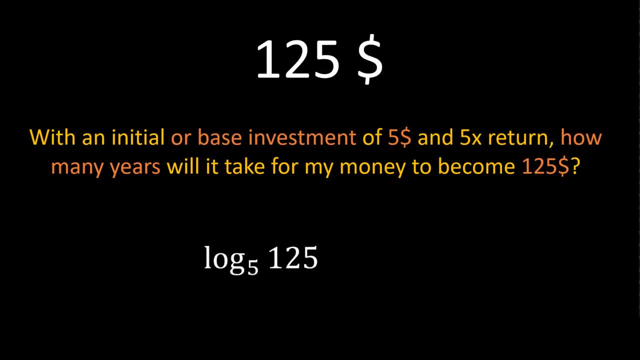 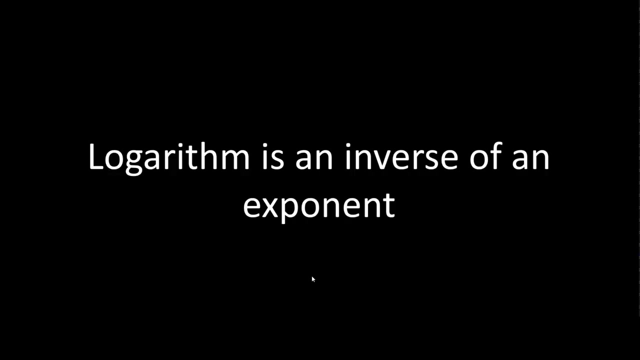 Well, that answer can be given by log function. So log to the base 5, because I started with base investment of 5.. $125 is the amount I have today and that can tell me that it takes 3 years. So you see, log is basically a reverse or an inverse of an exponent function. It tells you 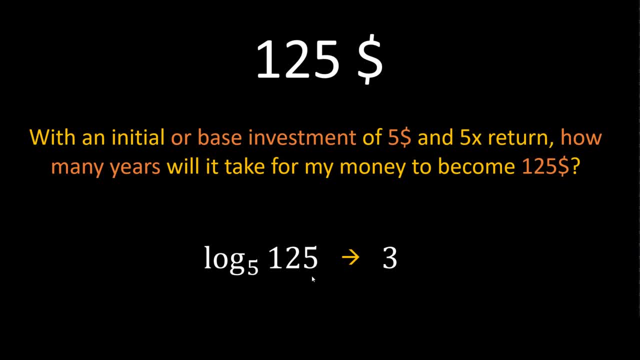 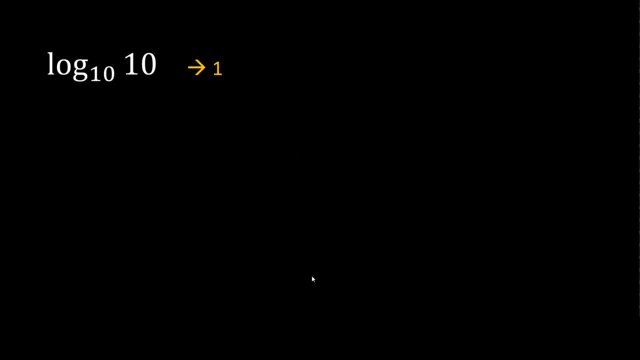 $125 is a given amount, How many years will it take for your base amount, which is $5, to become $125?? And the answer is three. The popular log is log to the base 10, and log 10 to the base 10 is one. 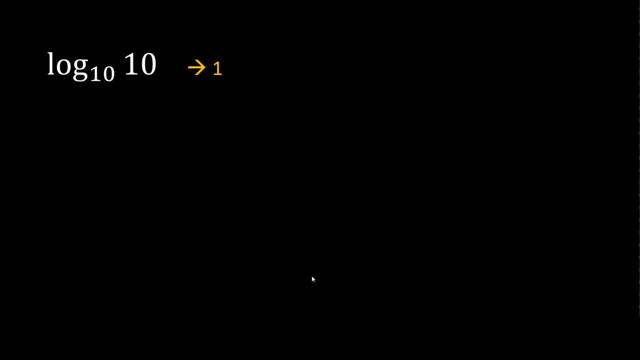 In general, log x to the base x is one. You have to remember this formula. If you have log 100 to the base 10, that can be written as this: and then 2 comes in the front and you already know log 10 to the base 10 is one. So this becomes: 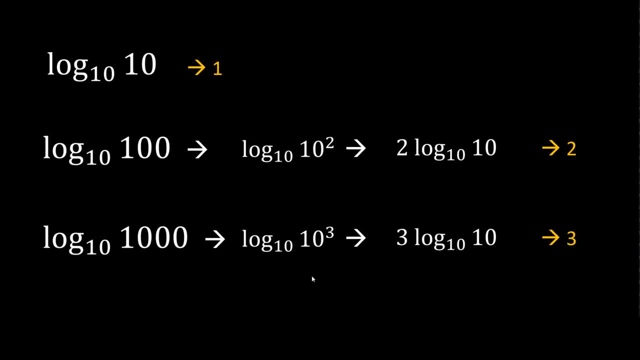 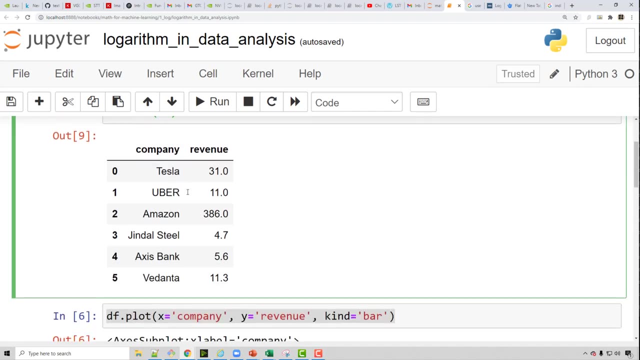 two similarly log 1000 to the base 10 is 3.. now let's see how log can be used in the data analysis process. so here i have downloaded uh company's revenue into my pandas data frame. i have six companies and these are the revenues. for example, amazon has 386 billion dollar a year. uber has 11. 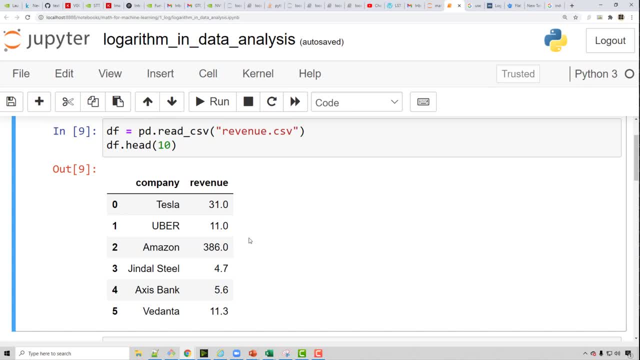 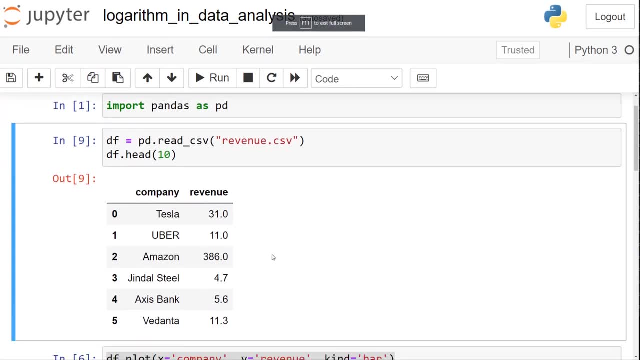 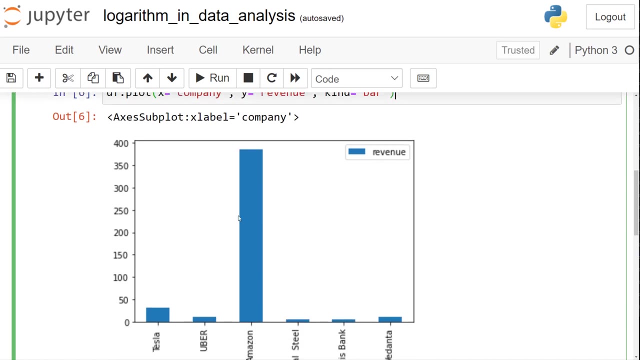 and so on. now, if i want to compare revenues using a bar chart, you know which is what people normally do- they use bar chart or different kind of charting visualization for doing data analysis. so here i am using, you know, by bar chart for comparing the revenues, and what i will notice is since 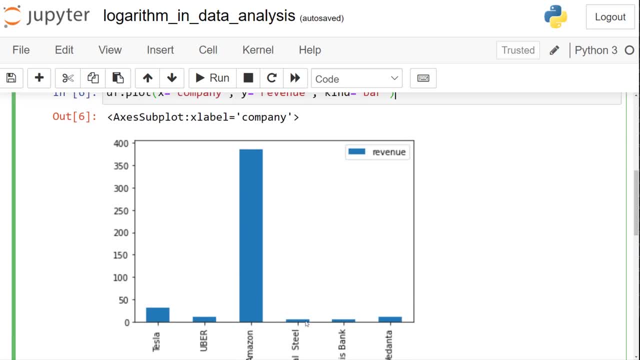 amazon's bar is so high it is almost flattening the smaller bars. so here i'm having hard time comparing jindal, still an axis bank, because the bars are almost looking same. see, you see only one big bar, everything else is kind of similar. log axis solves this comparison problem. so if you want to, 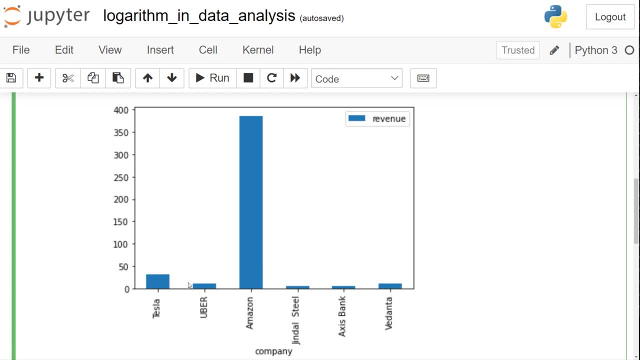 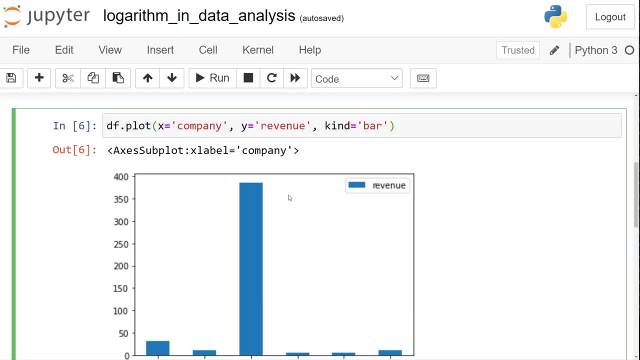 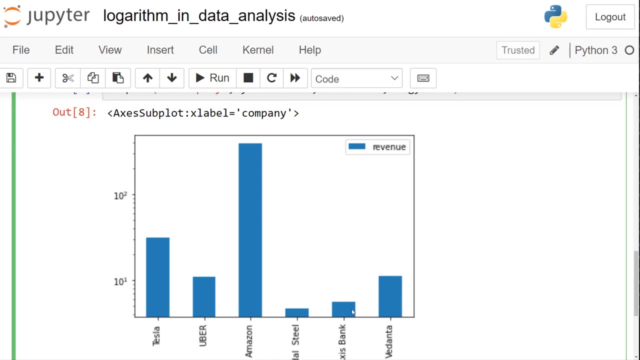 do comparison of all these smaller players in a better way. you can run the same function, dfplot, same, exactly same function, but you supply additional argument called log. y is equal to true and you get this as a result. now you see, the bars are little comparable here. i can at least say jindal still's revenues are less than axis bank. 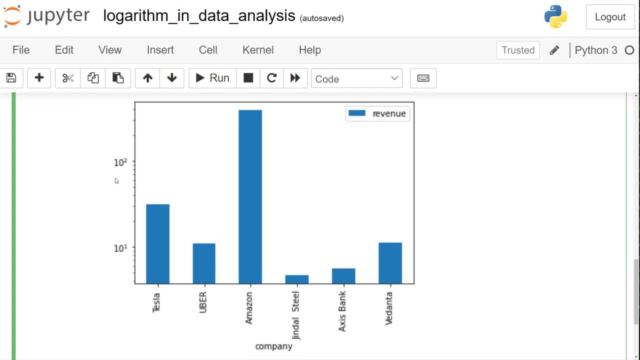 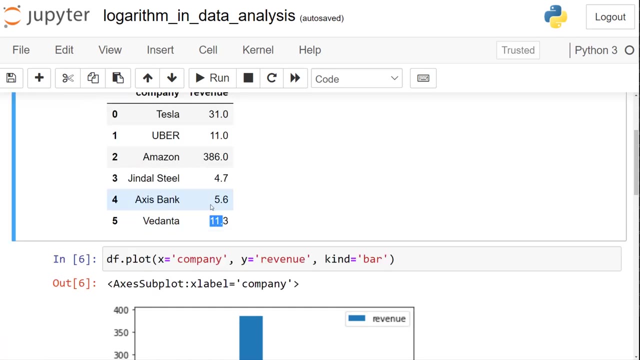 axis bank is close to five. you see this is 10, this is 100. so here axis bank is close to five. jindal still is little less than five. vedanta is more than 10. so you see vedanta is what: 11, x is 5.6, 4.7 and so on. so using log axis you can do better comparison when you have. 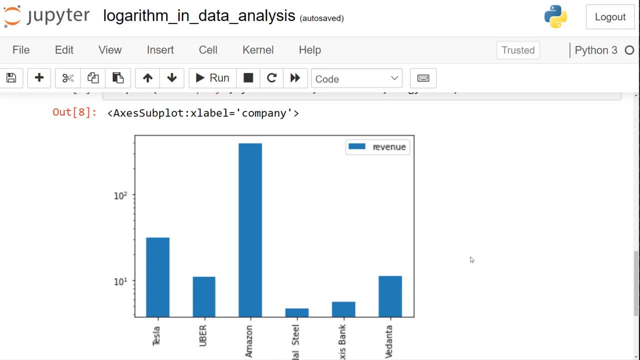 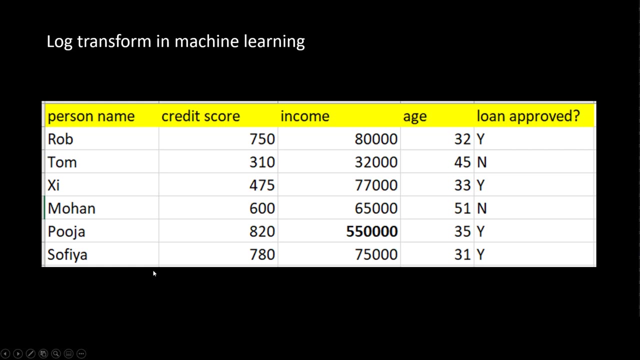 some values which are very high and other values are in every scale. so you will see people using log axis on occasions like this a lot in the jupiter notebook when you're performing your data analysis. another use case of log is using log transform in machine learning. 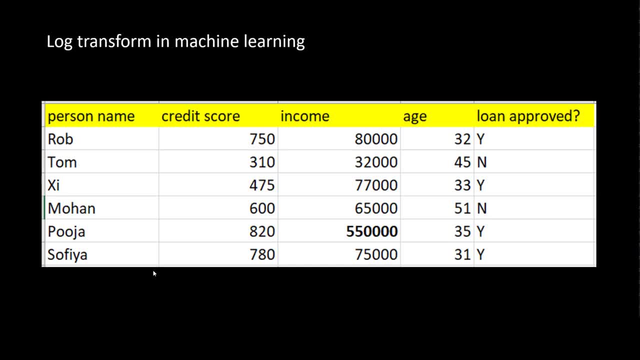 here is a classical problem of predicting if a loan should be approved for a given person. for a person, there are different features, such as credit score, income and age, and based on these three columns, you are deciding if loan will be approved or not. and this is a standard supervised learning problem. now, if you notice income column, 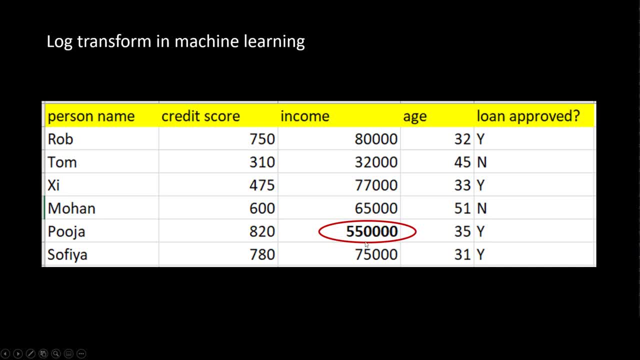 here you will see that pooja's income is very, very high: five hundred fifty thousand dollar a year, versus all other players are thirty two thousand seventy seven thousand dollar a year. so you have this one data sample, which is very high income. you you might have couple of such samples and when you 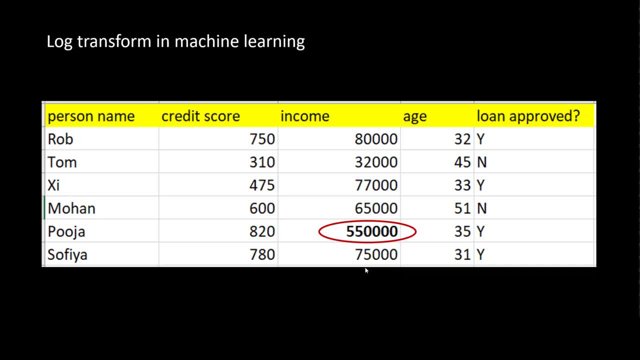 train a machine learning models. what happens is, because of the magnitude of this data point, it will negatively influence your model. so basically, your machine learning model will be biased, you know. so to solve this problem you can create a new column called log income. so you see the last column here and that. 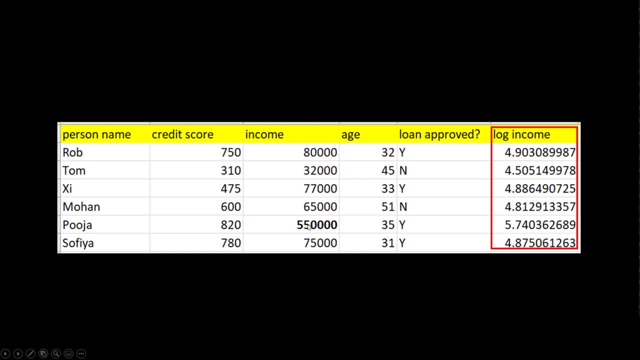 will be a simple log of this income. so log to the base 10 of this column gives you this. now here you can see that log income is 5.7 and rest of the people are 4.8- 4.5, so log will bring all these. 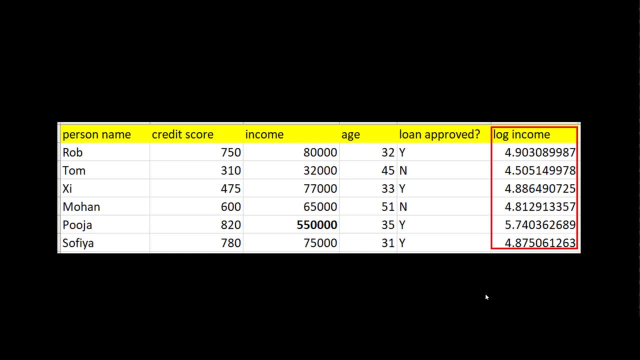 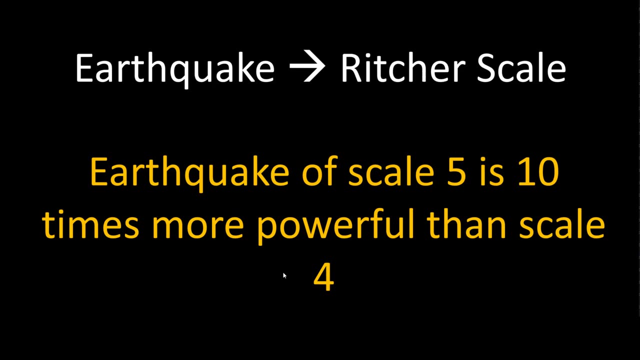 values on more comparable scale so you can compare these values in a better way. and when you train machine learning model using these comparable values, the model will not be biased and it will give you more accurate results. earthquake measuring. earthquake is another classical example of function. here, when you are comparing, let's say, earthquake five versus earthquake four, you can 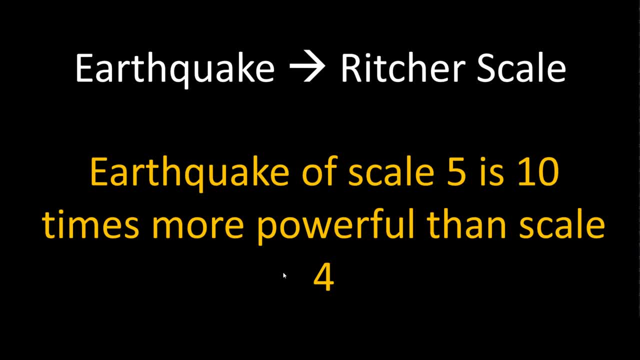 tell one thing immediately, which is earthquake of scale five is ten times more powerful than scale four. so if you're living in california, if you're going through earthquake and you know if it is four versus five versus six, six is very, very high. so five is ten times more powerful than four.